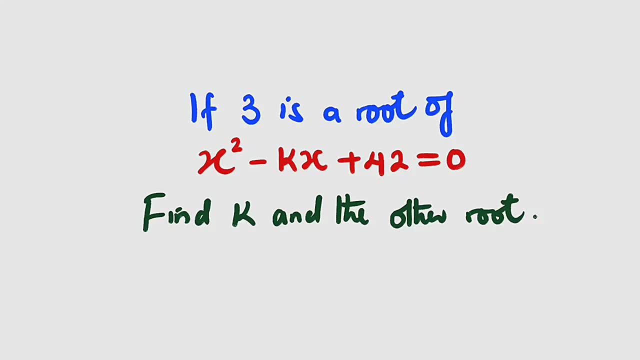 Hello, good day viewers. In this tutorial, we are going to find a solution to this problem, which I have posted on my Facebook page. The question reads: if 3 is a root of the quadratic equation, x squared minus kx plus 42, equal to 0, we 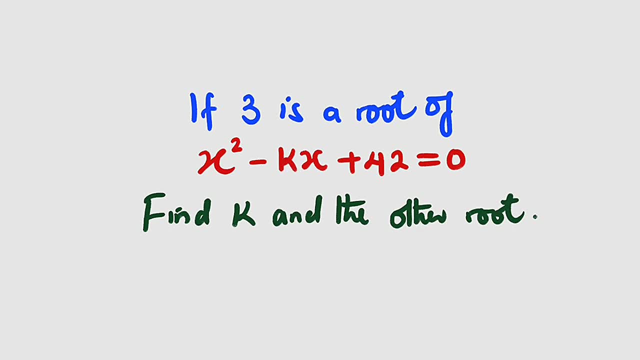 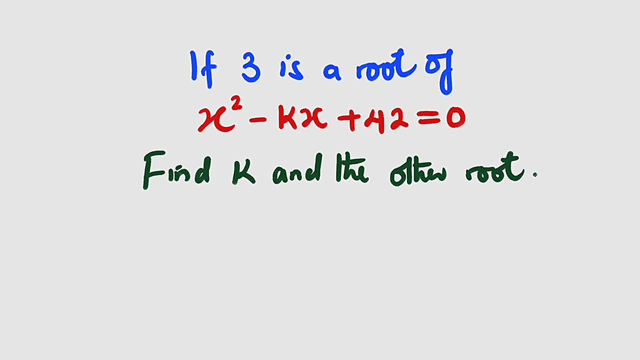 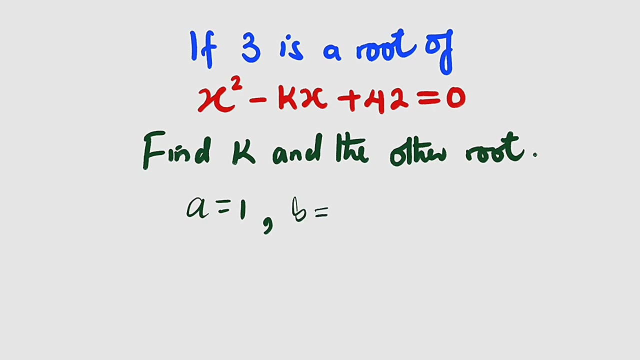 are asked to find the value of this k as well as the other root, because you know, a quadratic equation is expected to have two roots. Alright, let's get started. The leading coefficient is 1, so a is equal to 1.. b is the coefficient of x. 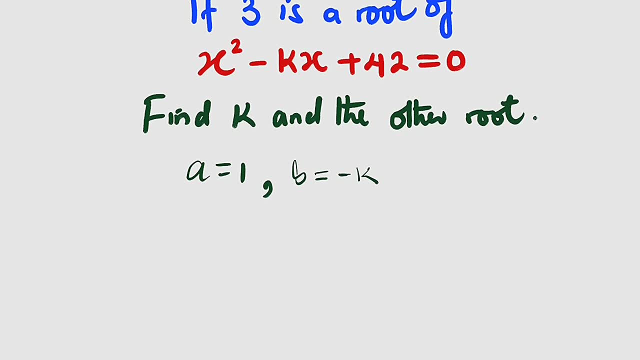 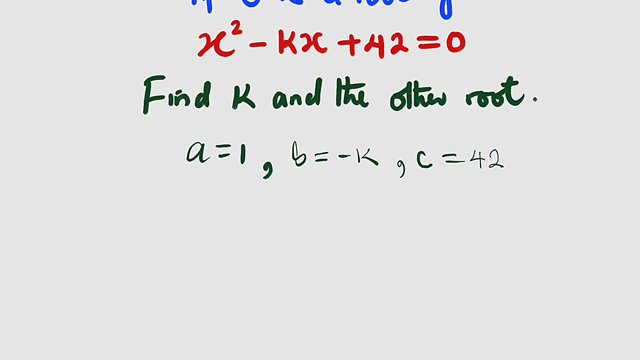 which is negative k. Then the constant c is what 42.. Let alpha and beta be the roots of this quadratic equation. So what will be the sum of alpha and beta? It is given as: what Minus b divided by a. Then 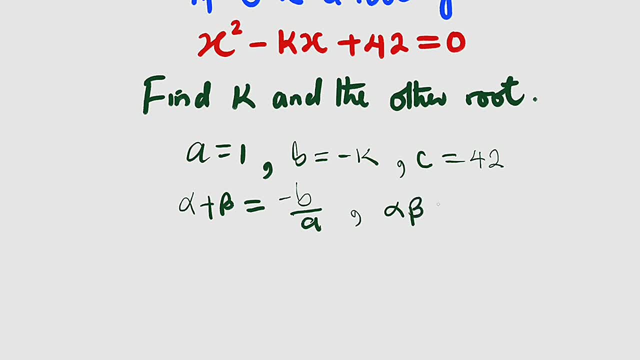 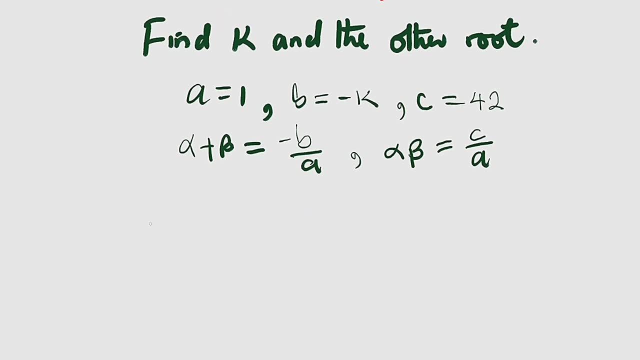 the product. if you multiply them together, alpha multiplied by beta is the same thing as c divided by a. Alright, so let's find them. Alpha plus beta is equal to minus b. What is b? b is negative k, So we have negative, negative k divided by a. 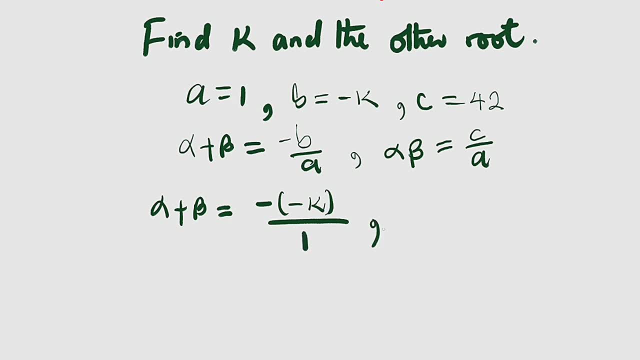 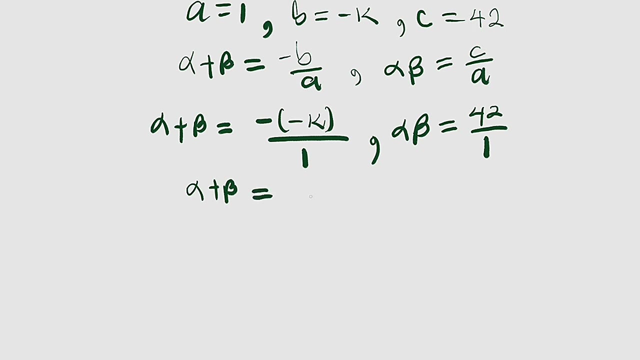 which is the leading coefficient, is 1.. Then, for the product, alpha beta is equal to c, which is 42, divided by a, which is 1.. Let's simplify: We have alpha plus beta equal to negative, negative, k is positive. k divided by 1 is k. Then 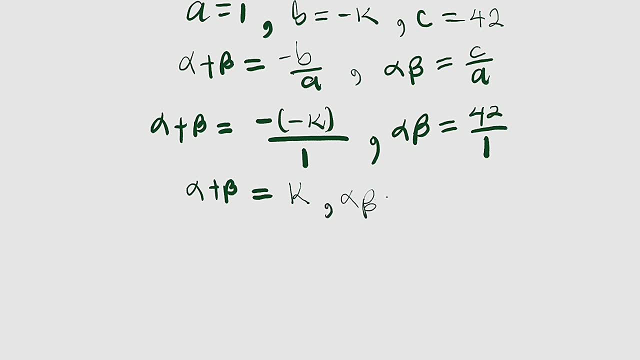 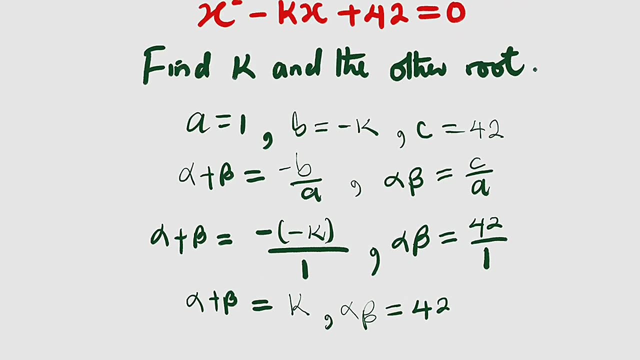 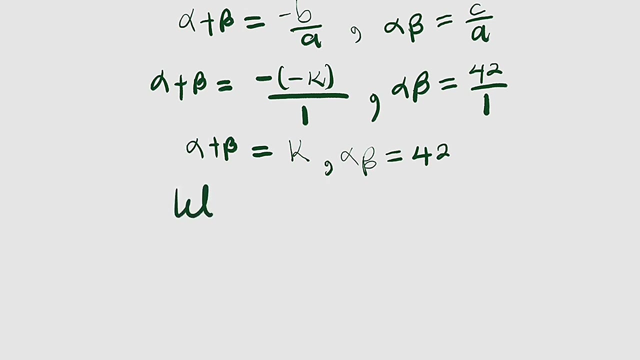 alpha multiplied by beta is equal to 42 divided by 1, which is still 42.. Alright, but remember, one of the roots is given as 3.. So we can choose any one of them. Let's choose alpha to be equal to 3.. Let alpha be. 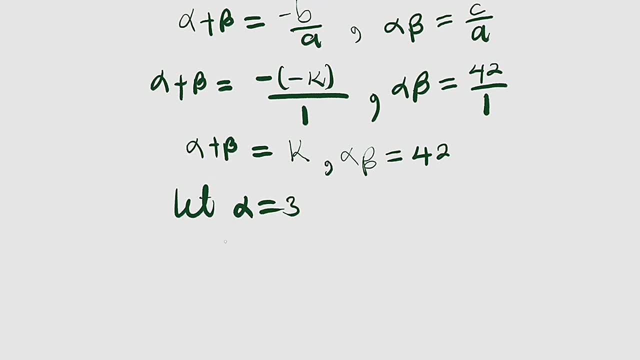 equal to 3.. So we have 3 plus beta. we are looking for beta. 3 plus beta is equal to k, and 3 multiplied by beta, 3typled by beta, is equal to 42. So let's find beta from this equation. It.